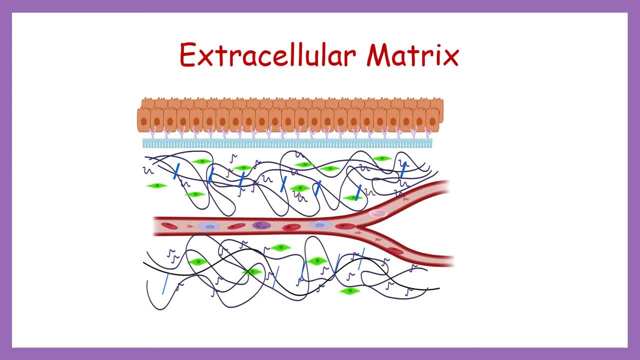 Let's start with the extracellular matrix. Extracellular matrix made up of basement membrane and the interstitial matrix. The basement membrane has a mesh like structure and present between the epithelial cells and the underlying connective tissues. It's strongly cross-linked comenent of ECM that made up of sheet and toughest tissue very similar to Habits membrane. So adventuring into the complex to try and destroy extracellular cells. So that's the important point Before Friday. we note that the base membrane has its primary footprint and portion of NE3 which is shown in the video. All the cyt Seongate. 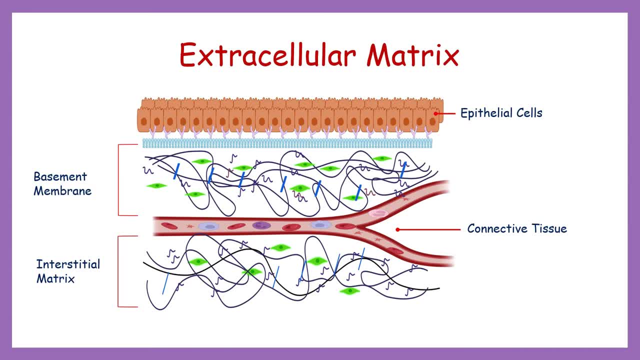 like deposition which is released by epithelial cells In every given tissue. the basement membrane divides the epithelium from the stroma. It is constantly in contact with the cells, which provides structural support, dividing tissues into compartments and regulating cell behavior. Interstitial matrix contains large amount of collagen or laminin proteins. They also contains 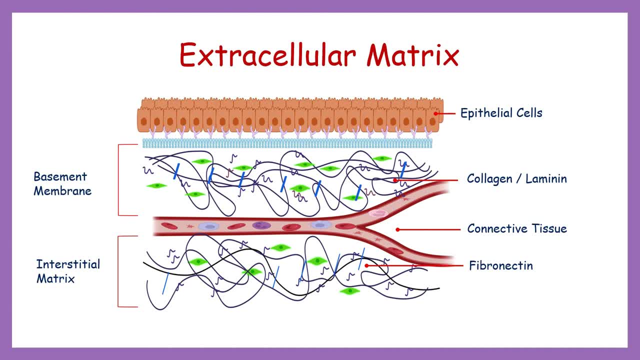 glycoproteins like fibronectin, glycosaminoglycans, which include heparin, sulfate, high aluronone, proteoglycans and various growth factors like transforming growth factor beta. These matrix also contains other secreted proteins like proteolytic enzymes and protease inhibitors. 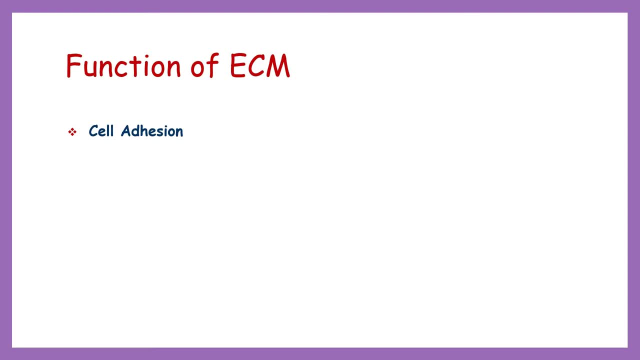 The fundamental purpose of the extracellular matrix is to aid cell attachment and communication with or adjacent cells. It also plays a role in cell growth, proliferation, mortality and differentiation into other specialized cells and cell signaling. If the component of the ECM are altered, as a result, various diseases such as fibrosis, cancer and 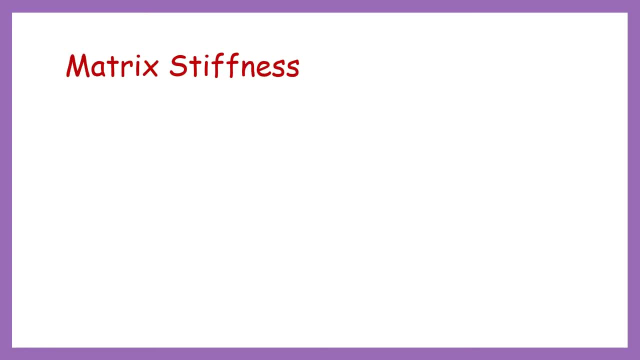 genetic problems would follow. From the delicate tissues of the brain to the hard tissues of the bones, the ECM can have different stiffness and elasticity levels. The ECM elasticity can vary by several orders of magnitude. This feature is primarily influenced by collagen and elastin. 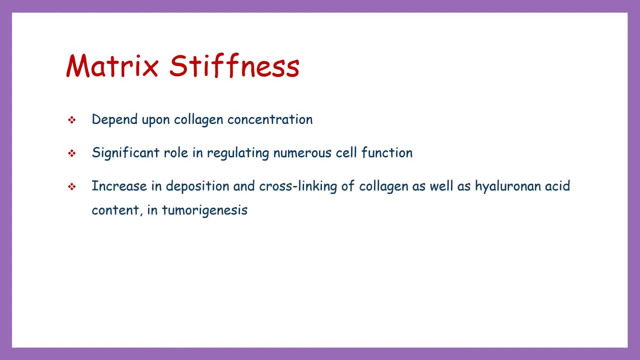 levels, and it has recently been discovered to play a role in controlling a variety of cell processes. When it comes to tumors, they are frequently stiffer than surrounding healthy cells, Due to an increase in collagen deposition and cross-linking, as well as high alluronan. 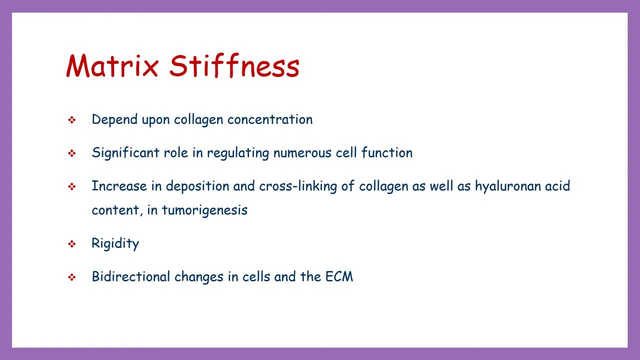 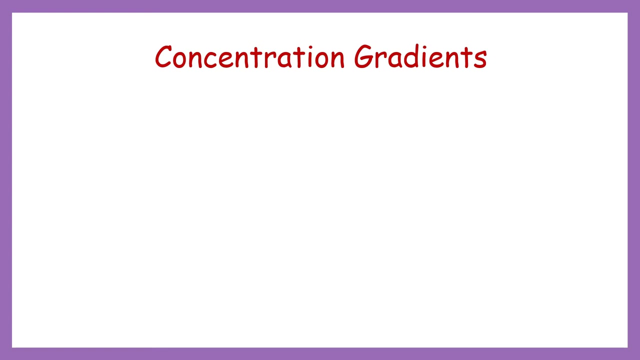 acid concentrations. ECM stiffness has also been linked to tumor growth in the past. Physical cues like stiffness often vary in tandem with changes in ECM composition, resulting in bidirectional changes in cells and the ECM Within a tissue concentration. gradients exist for oxygen, pH nutrients, effector molecules as well as cellular metabolites. 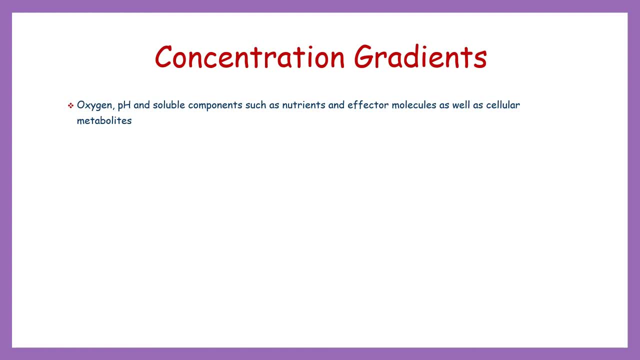 These natural gradients are influenced by the proximity to blood vessels, by the diffusion of molecules through the ECM. Yes, ECM is important to exchange or to regulate the oxygen and nutrient consumption with the cells and the production of cellular waste products. also, Molecular concentration gradient affect various cell behavior. 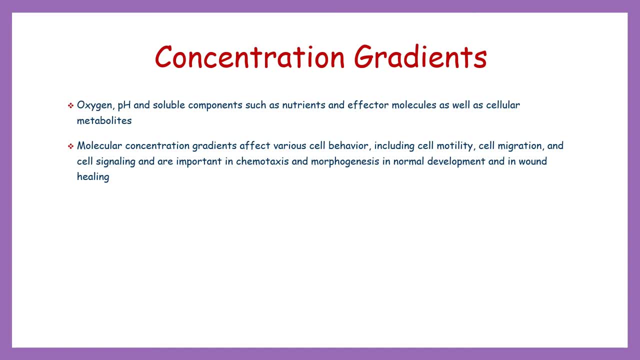 including cell motility, cell migration and cell signaling, and are important in chemotaxis and morphogenesis, in normal development and in wound healing. If we talk about the tumor 3D tumor, spheroids are much more representative of IV tumors. 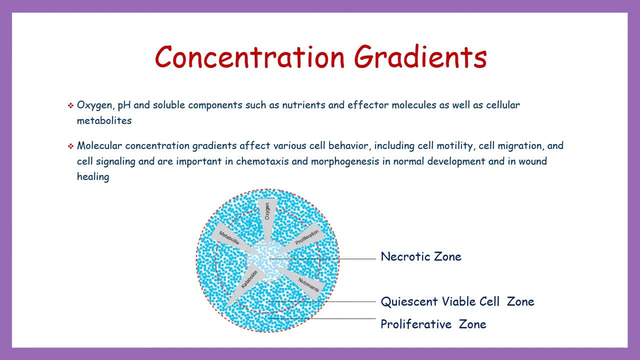 There is peripheral layer having proliferative cells due to the closeness to the supply of oxygen and nutrients, underlaid by an intermediate layer having crescent cells and an inner necrotic core. This wear can mimic inward diffusion to form oxygen and nutrient gradients and a perfect 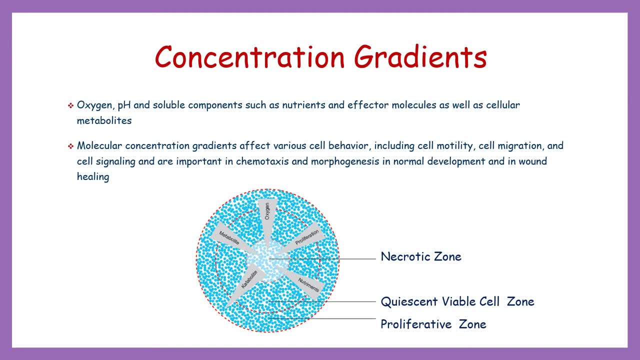 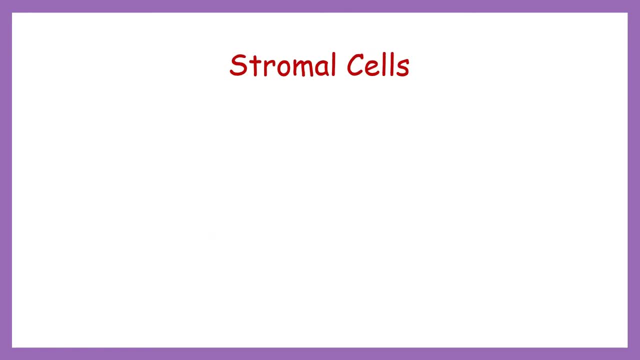 model for in and outward diffusion of regulatory molecules and provide a reservoir for the accumulation of waste. Another thing: we should know that in vivo, cells are not only surrounded by ECM and ECM associated signaling molecules, but connective tissues also contain stromal cells, including. 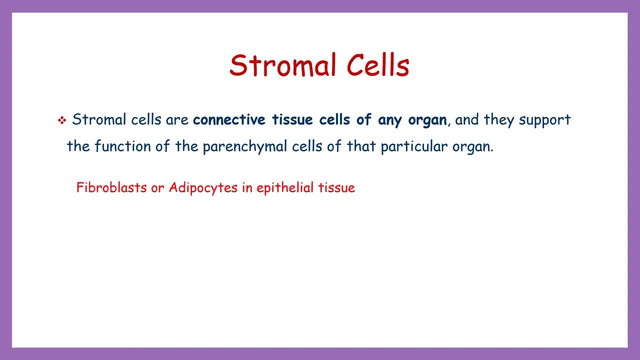 mesenchymal supporting cells such as fibroblasts or adipocytes in epithelial tissues, glial cells in neuronal tissues, cells of the surrounding vasculature and cells of the immune systems. Interaction with stromal cells can regulate surrounding epithelial and neuronal tissue. 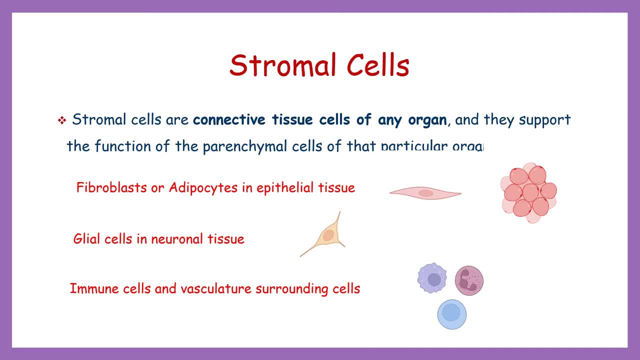 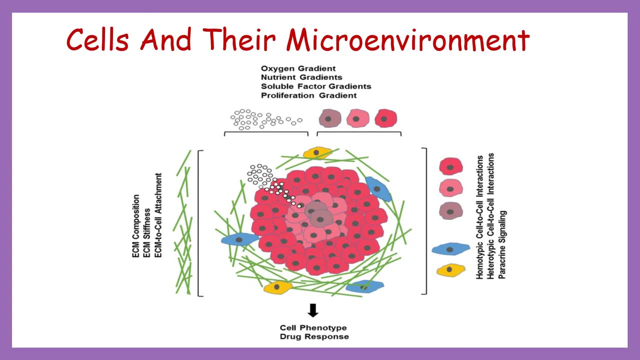 which contribute to disease prevention In living tissues. cells exist in 3D macro-environments with intricate cell-cell and cell matrix interaction and complex transport dynamics for nutrients, oxygen, soluble factors and cells. Standard 2D or monolayer cell cultures are inadequate representation of this environment. 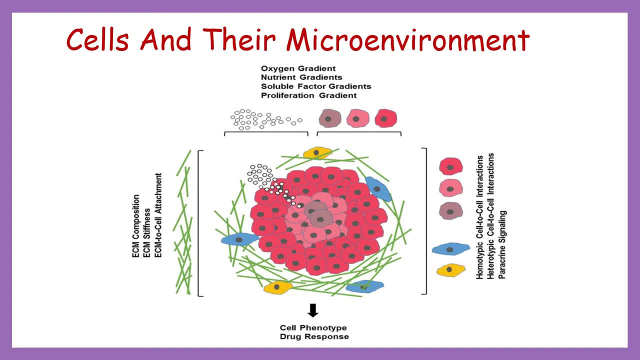 which often makes them unreliable predictors of the environment. Instead, it is Enough to be a溶-free cell. 3D. spheroids more closely resemble in vivo tissues in terms of cellular communication and the development of ECM. These matrices help the cells to be able to move within their spheroids similar to the 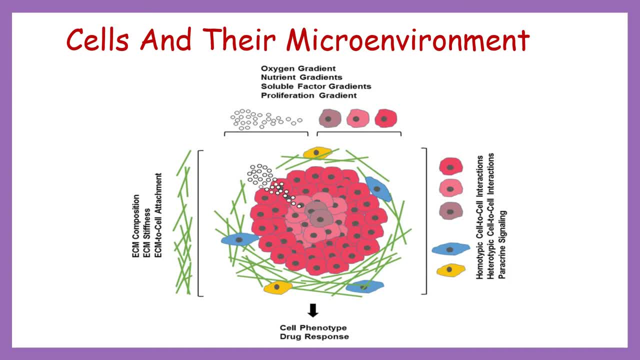 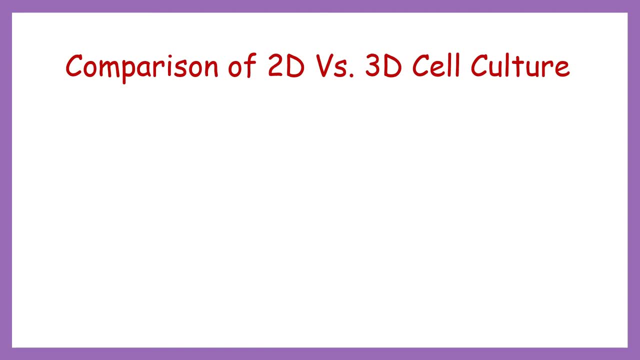 way cells would move in living tissues. The spheroids are thus improved models for cell migration, differentiation, survival, health and care and growth. Now let's compare the 3D cell culture with 2D cell culture In 3D cell culture system. 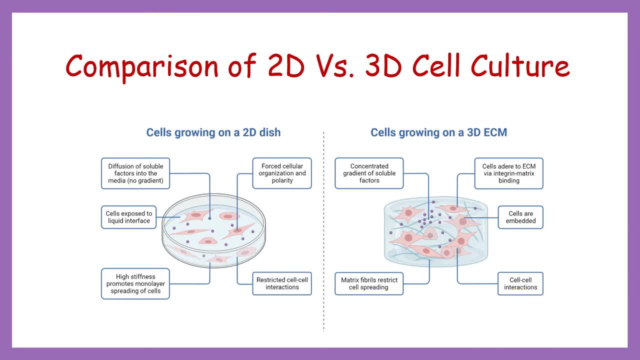 cells will allow to grow in 3D environment, where cell-cell and cell matrix interaction occurs, whereas in 2D cell culture system cell-cell interaction is restricted and cell matrix interaction is absent. In 3D cell culture there is a gradient for nutrients, oxygen, pH and others. 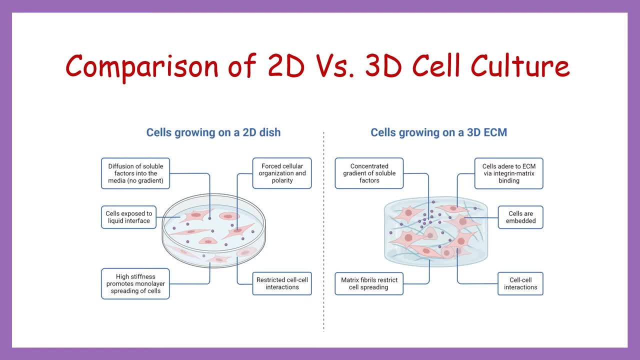 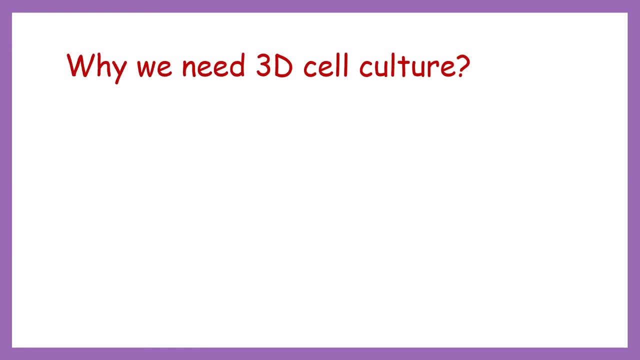 as we talked previously, In 2D cell culture, gradient mechanism is totally absent. In 2D cell culture system, cells exposed to liquid interface, whereas in 3D cell culture system, cells are embedded. It's now evident why we need 3D cell culture, If you think about it. 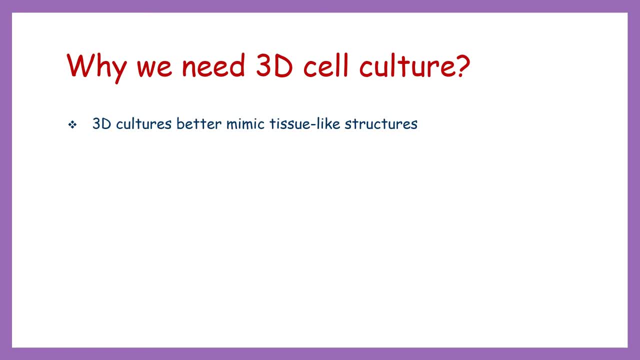 no cell types within our body grow as a monolayer or independent of other cells or tissues. Instead, most cells are not monolayer. In 3D cell culture system, cells are not monolayer. Most cells naturally exist in complex 3D structures including different cell types. 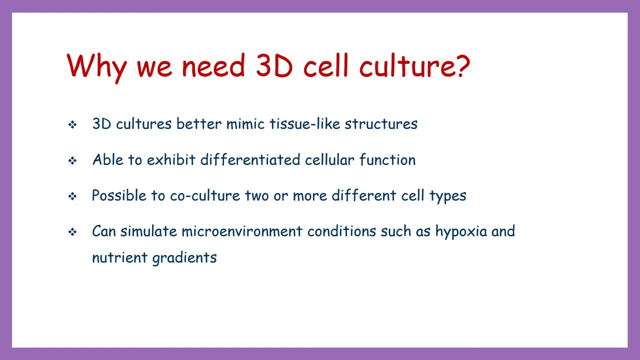 within an extracellular matrix. The numerous cell-cell and cell matrix interaction all have a profound effect on their behavior and there is a possibility to co-culture two or more different cell types. In 2D monolayer there is a uniform access to nutrients and oxygen, which is not the case in tumors. In 2D monolayer there is a uniform access to nutrients and oxygen, which is not the case in tumors. Given theof three different cells in foods, we propose different guerrillas to develop different threat strategies that test the four different cells. 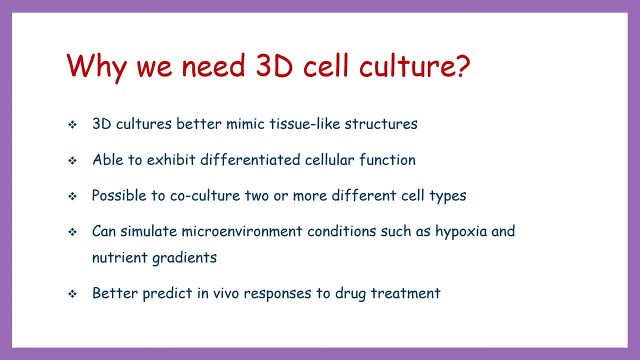 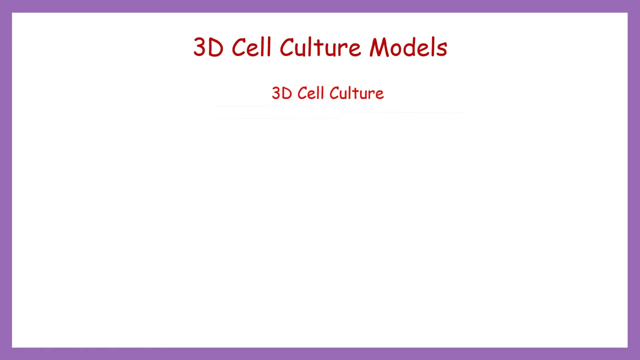 As we talk about in previous slides. 3D tumours upwards are much more representative of in vivo tumours, in which inner cells have less access to nutrients and oxygen compared to the outer layer, because they all form a natural gradient. Now lets talk about 3D cell culture models. They have been divided into 3 categories. 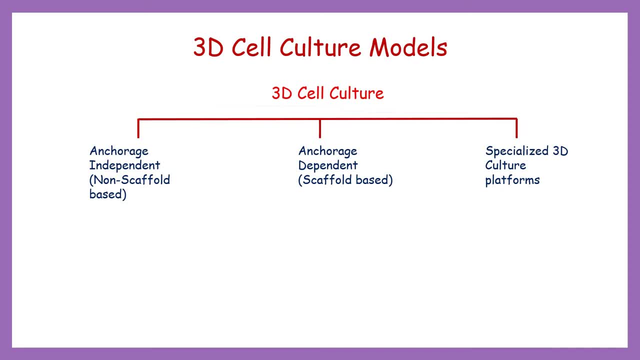 that is also called non-scaffold based. second is anchorage dependent, also called scaffold based, and third is specialized 3d culture platforms. anchorage independent includes two techniques. first is hanging drop and another is low attachment plates. anchorage dependent, which is scaffold based, includes hydrogel technique, which is divided into biological and synthetic. 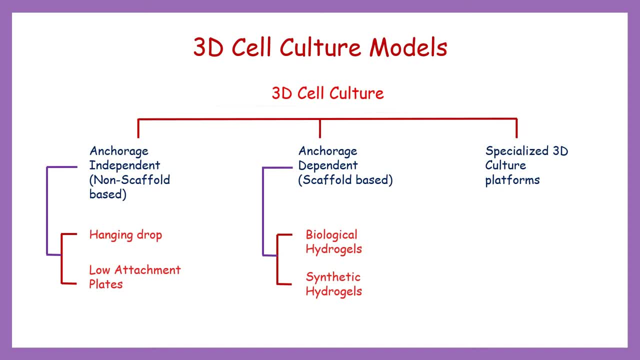 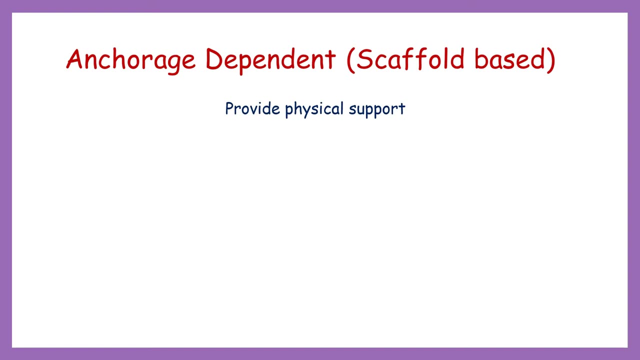 hydrogels. specialized 3d culture platforms includes macro fluidic devices and micro patterned plates. so now let's learn these techniques in details. scaffold based culture technologies provide physical support, ranging from simple mechanical structures to ecm like matrices on which cells can aggregate, proliferate and migrate. 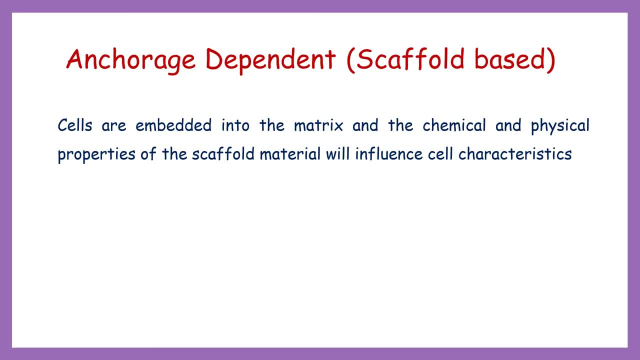 in scaffold. scaffold based 3d cultures. cells are embedded into the matrix and the chemical and physical properties of the scaffold material will influence cell characteristics. scaffold can be of biological origin or they can be synthetic, engineered to mimic key properties of ecm such as stiffness, charge or adhesive moieties. in some synthetic scaffolds, growth factors such as adhesion 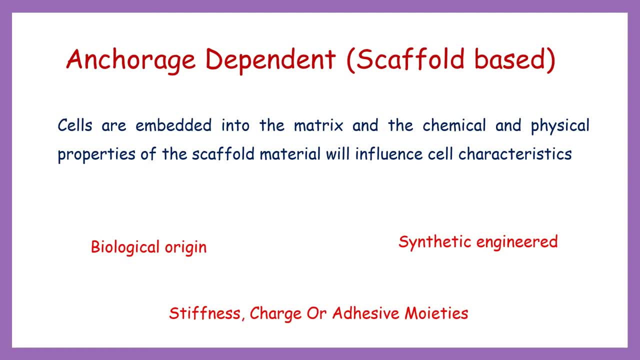 or adhesion of the material will be affected by scaffold based 3d cultures. cells are embedded in scaffold based 3d cultures. cells are embedded in scaffold or biome, an under suspension or corrective segmentation of the structure along the scaffold and the left side of the scaffold. 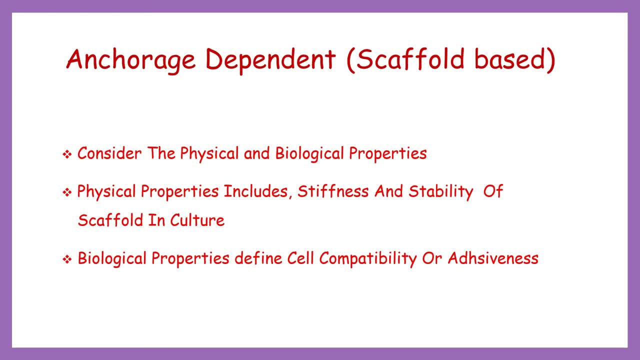 will be affected by effect of the moisture formation in multiple cells, while the right side of scaffold can be used for specific structure, like a barb and a drop or a pinch, or it may be all or a few other factors. factors, hormones or other biologically active molecules can be encapsulated to enhance cell. 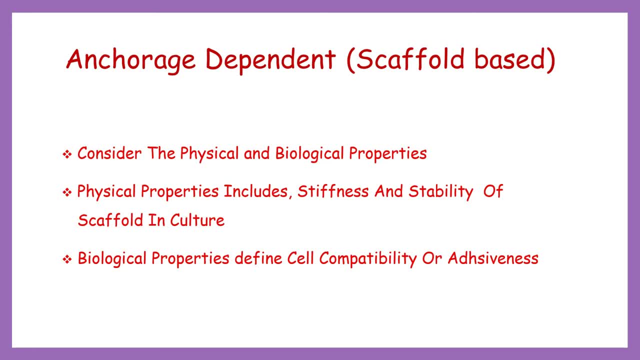 and biological properties define cell compatibility or adhesiveness. Hard polymers can provide the physical support found in a specialized tissue, such as skin, tendons or bone, and micropattern surface. microplates can be designed for specific application, such as support of cell networking. 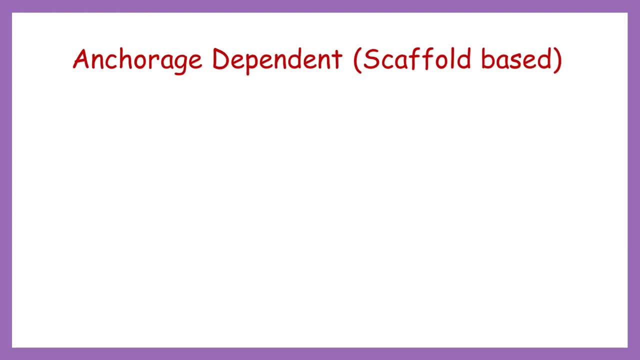 Hydrogels are networks formed from dilute polymer chains with given structure and properties obtained either by intermolecular or by interfibrillar cross-links. Although hydrogels display solid-like material properties in a quiescent state with over 95% of water by volume. 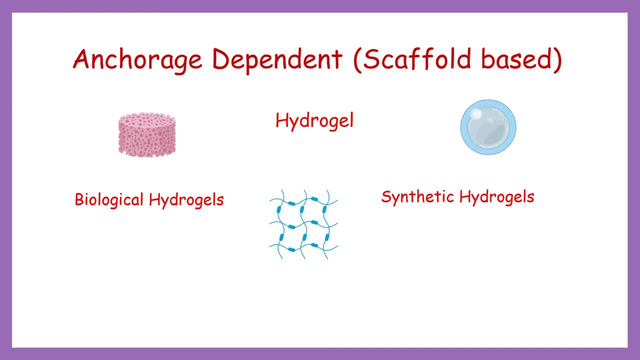 they can indeed provide a cell-liquid interface. Hydrogels may correspond. They can come from natural sources or can be synthetic, with the possibility of mixing different hydrogel materials to obtain hybrid hydrogels possessing new physical and biological properties. Hydrogels from natural sources, such as collagen, metragel, are biocompatible. 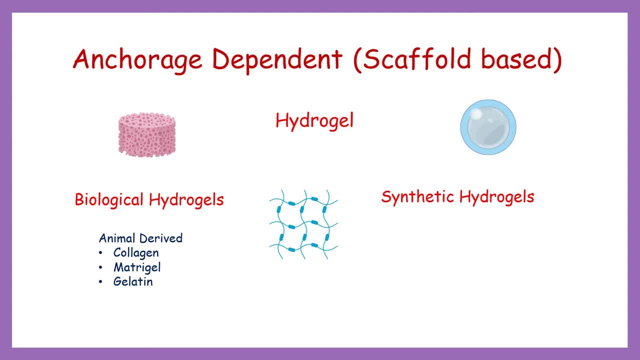 have natural adhesive properties and sustain many physiological cell functions, resulting in high cell density. Hydrogels can be used in the treatment of various cell viability, controlled proliferation or controlled differentiation, and often as cell phenotypes typically observed in vivo. 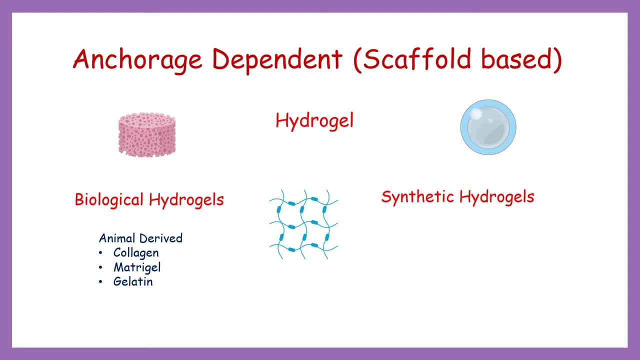 Collagen, with type I collagen being the most abundant form, is the most widely used ECM protein for 3D cell culture. Gelatin is a partially thermally and chemically degraded product of collagen and can be stabilized by a covalent modification. 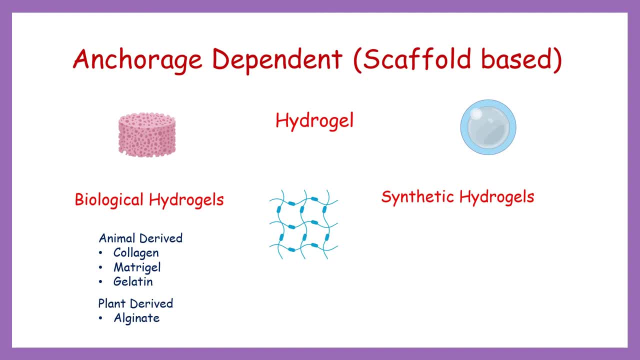 The possibility of covalent linking of functional groups also allows for the production of specialized gelatine gels. Another natural hydrogel is alginate that is isolated from the cell walls of brown algae. The mechanical properties and rapid degradation of the alginate hydrogel somewhat limits its application for 3D cultures. 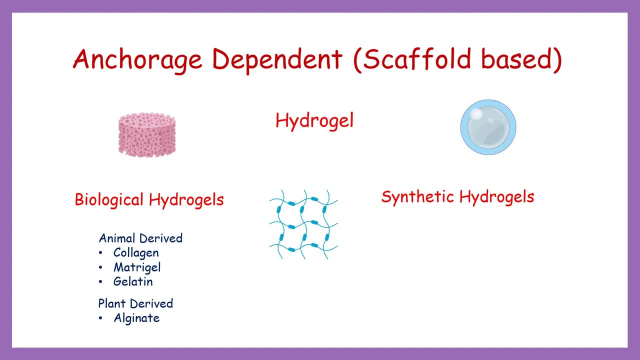 But alginate hydrogels have found their place in the cell walls of brown algae. But alginate hydrogels have found their place in the cell walls of brown algae. Alginate hydrogels have found their use as 3D printed scaffolds for specialized tissues such as vascular tissue, bone and cartilage. 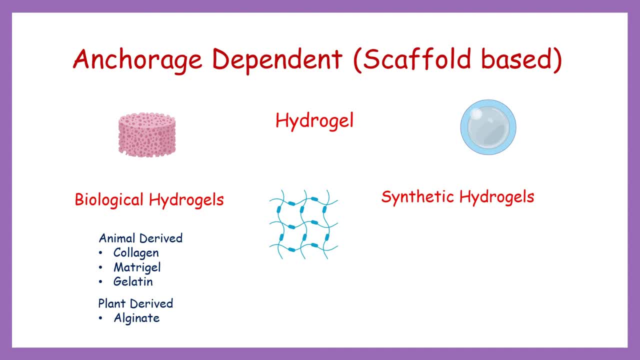 When well-designed synthetic hydrogels are ideal material to use as 3D cell culture scaffolds, as they can mimic biological properties of ECM and be functionalized with defined adhesivoides that include proteolytic sites and encapsulate growth factors. 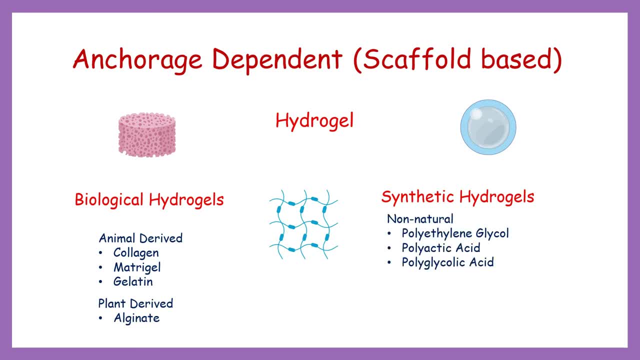 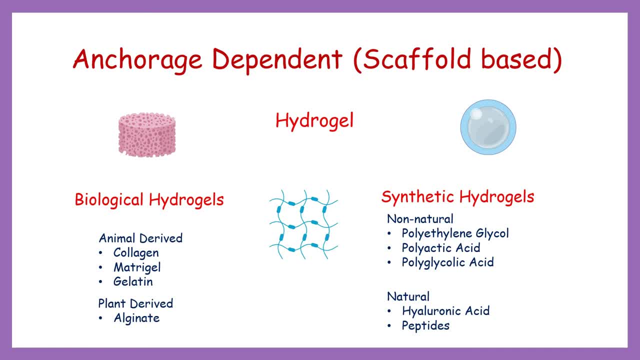 Polyethylene glycol, poly-ylactic acid and poly-ylactic acid are the main components of synthetic hydrogels linking and are more reproducible, thereby supporting the acquisition of consistent results. On the other side, unnatural polymers lack adhesive moieties found in natural ECM and 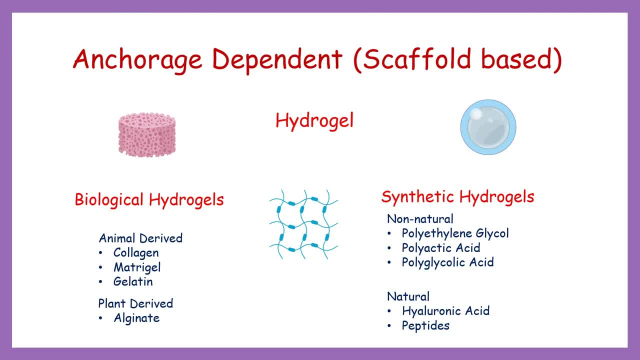 require cross-linking of biological peptides to the scaffold to improve functionality. Polyethylene glycol gels and their derivatives have been used in a variety of 3D cell culture applications, including stem cell differentiation, cell invasion and angiogenesis. Synthetic natural polymers share with non-natural polymers the advantage of consistent and tunable. 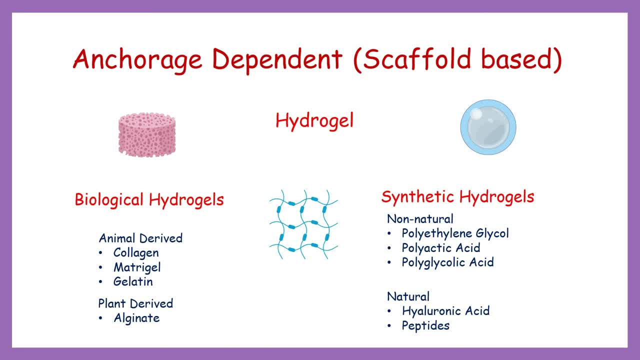 material properties for reproducible results. Due to the biological nature of their naturally occurring moieties, natural synthesized hydrogels are highly compatible with encapsulation of cells for 3D cell culture. However, material cost can be high due to complex chemical synthesis requirement. 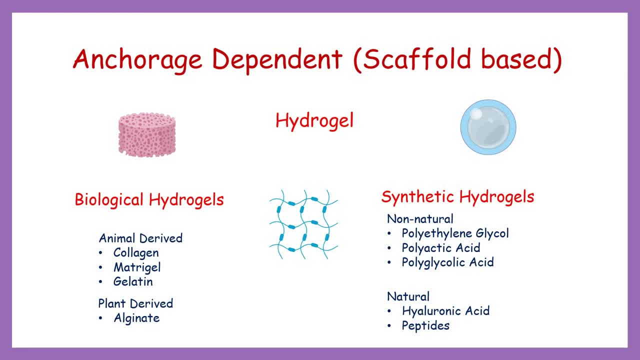 One of the best characterized natural hydrogel is high-aluronic acid, a glycosaminoglycane that can be modified with functional groups allowing for the formation of hydrogel with diverse properties for a wide range of applications. Small peptide-based hydrogel materials are an evolving field in materials science and 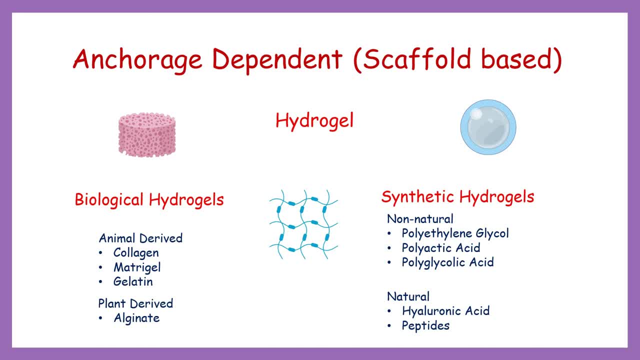 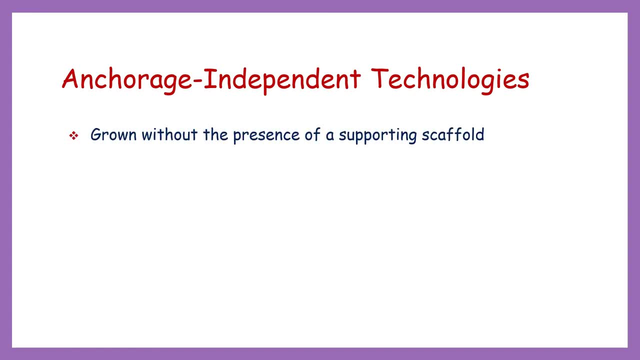 provide a new 3D cell culture. 3D cultures can be grown without the presence of a supporting scaffold, and that includes anchorage-independent technologies. Scephal-free methods depend on cells to self-assemble into clusters or spheroids. 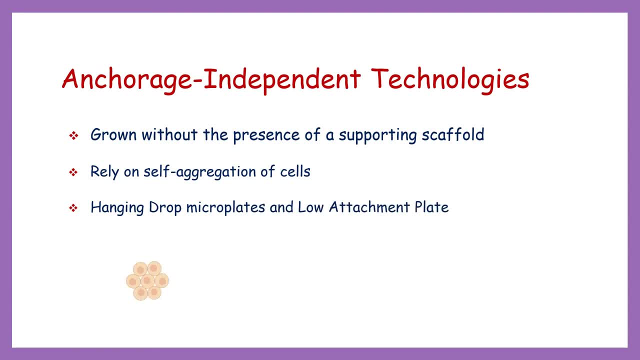 These spheroids are grown in specialized culture plates, which include hanging-drop microplates and low-adhesion plates with ultra-low attenuation. These microplates are also called spheroids. These are the most common types of spheroids. These spheroids can recapitulate physiological characteristics of tissues and tumors with 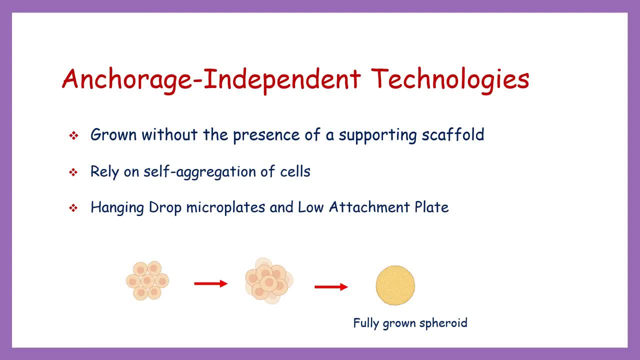 regard to cell-cell contact, and they can synthesize their own ECM, which can allow for natural cell-cell matrix interactions. Spheroid size depends on the initial number of cells seeded, and spheroids can be grown to a size where they can display oxygen and nutrient gradients similar to the size of a. 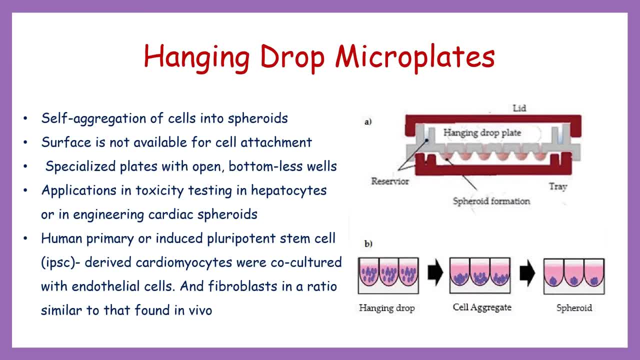 tissue Hanging-drop cultures are a well-known 3D culture technology taking advantage of cell aggregation of cells into spheroids. when a cell surface is not available for cell attachment, Hanging-drops can be created in specialized plates with open, bottomless wells that are 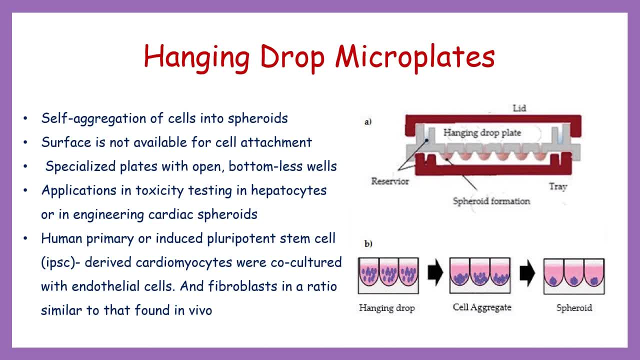 designed for the formation of a small droplet of media. The droplet is big enough for cells suspended in the media and it can be used as a thematic material for other types of cell growth. medium to aggregate, but small enough to prevent it from being dislodged during manipulations. 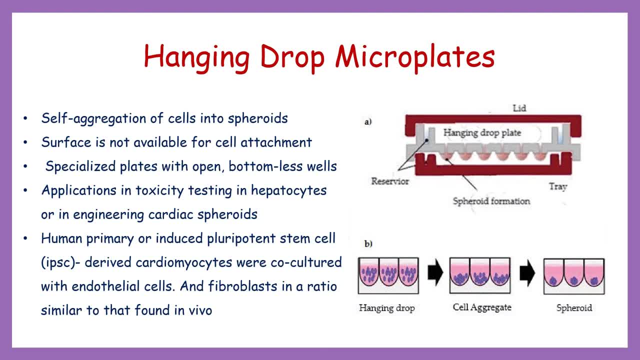 Hanging drop cultures have also found applications in toxicity testing in hepatocytes. In a recent study, human primary or induced pluripotent stem cells derived cardiomycetes were co-cultured with endothelial cells and fibroblasts in a ratio similar to that found in 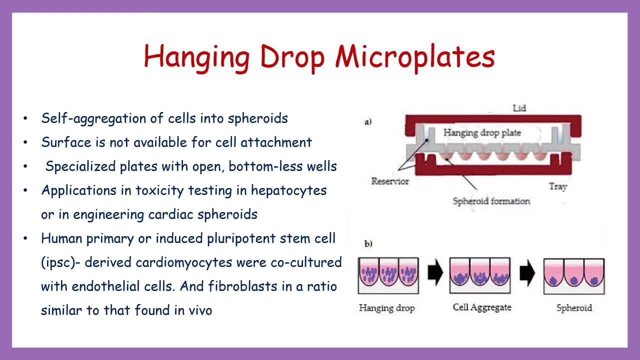 in vivo. The cardiac spheroid mimicked important in vivo features of the human heart, biochemically or pharmacologically, offering a 3D cell culture model to study toxic effects in human heart tissues. Similar to hanging drop plate cultures: spheroid macroplates with round, tapered or v-shaped. 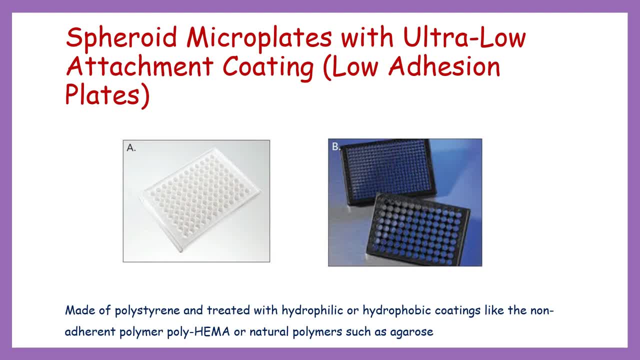 bottoms take advantage of the lack of cell attachment surfaces to promote aggregation of cells and spheroid formation. In contrast to hanging drop plate cultures, a transfer of spheroids to a different plate for prolonged culture or experimental procedure is often not necessary. Low-adhesion plates are often made of polystyrene and treated with hydrophilic. 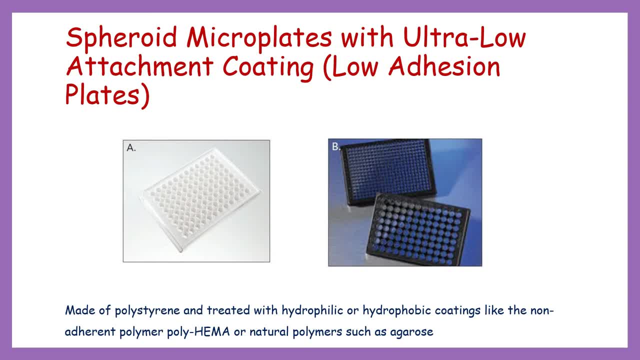 or hydrophobic coatings like the non-adherent polymer poly-HEMA or natural polymers such as agarose. The coating reduces the attachment of cells to the point that they preferably aggregate with each other to form spheroids Because of their larger volume. low-adhesion plates. 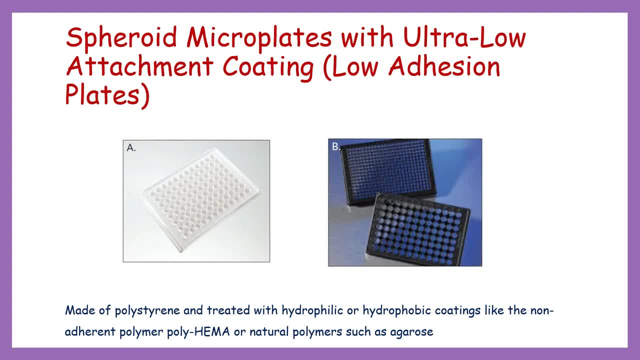 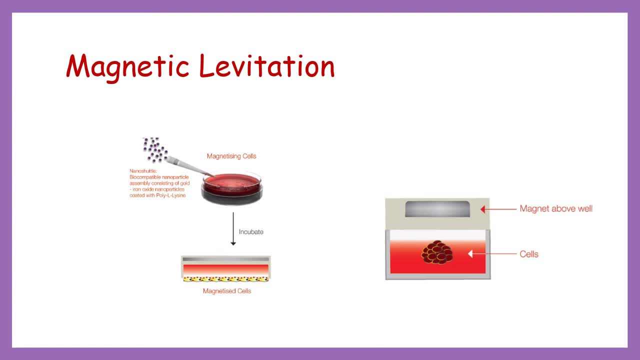 are well suited for multicellular culture and are frequently used for studies in tumor cells. Magnetic cell levitation is an emerging technique for the formation of spheroids. To generate spheroids, cells are pre-loaded to the spheroids. To generate spheroids, cells are pre-loaded. 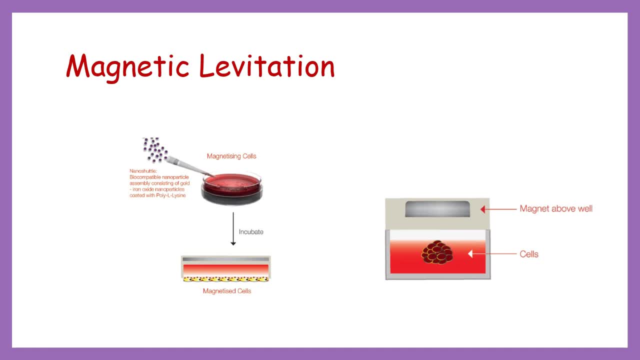 with magnetic nanoparticles and then, using an externally applied magnetic field, they are floated toward the air-liquid interface within a low-adhesion plate to promote cell-cell aggregation or spheroid formation. Magnetic levitation has been used to generate spheroids from cells of various tissues to form multicellular mesenchymal stem cells, spheroid and for tissue. 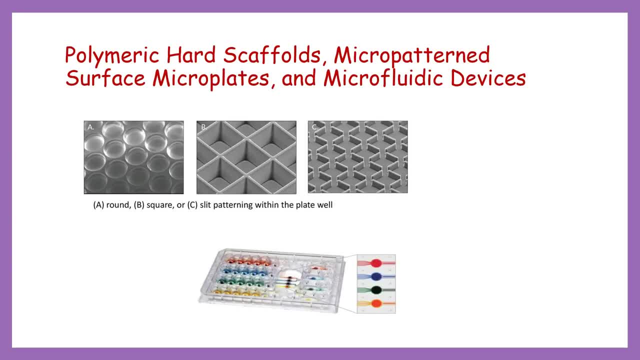 engineering. Microfabrication technology allows for the fabrication of an endless array of imprinted macro-patterns on the surface of plates. The micro-pattern plates are designed to promote cell-to-cell adhesion for scaffold-free macrosphere formation within the confinement of a macrospace. 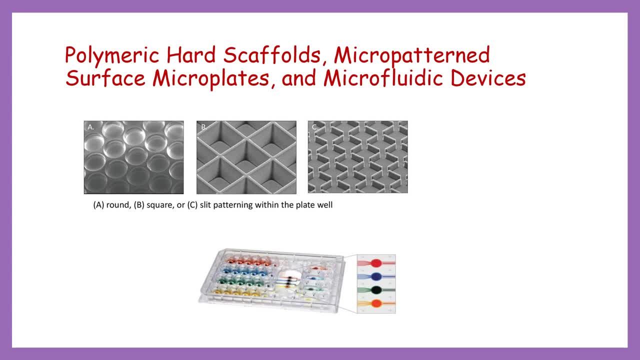 These plates are coated for low adhesion. Micro-pattern plates can also be manufactured to provide a scaffold-based three-layer adhesion Polymeric. pre-fabricated scaffolds such as porous discs, electrospun scaffolds or orthogonally layered polymers are physical supports that can be an inert matrix or designed. 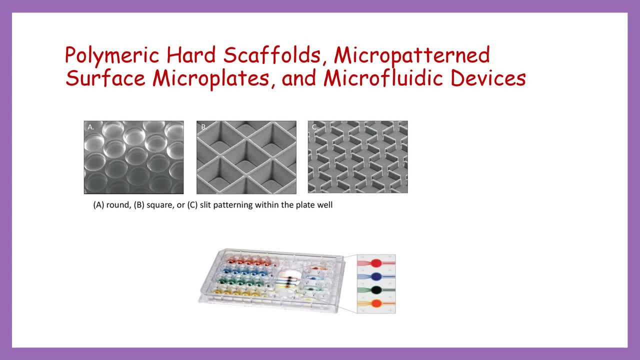 to mimic in vivo ECM on which cells can attach, migrate or fill scaffold compartments to form 3D cultures carrying a geometric configuration. Currently, the most common applications for such scaffolds are for tissue regeneration, re-creating the natural physical and structural environment of bone, ligaments and cartilage. 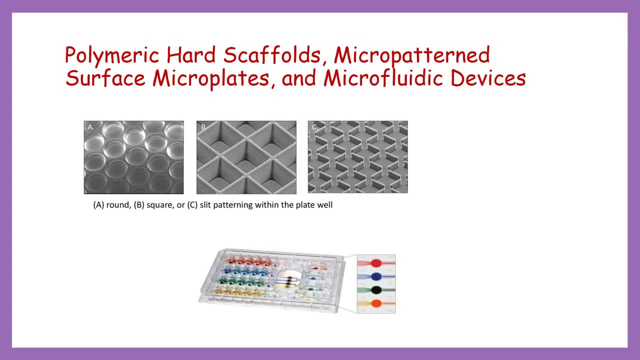 for skin, vascular, skeletal muscles or CNS tissue and for pre-clinical in vitro 3D culture testing for tumoroids or engineered tissues like organoids. On the other hand, micro-fabricated scaffolds such as porous discs, electrospun scaffolds. 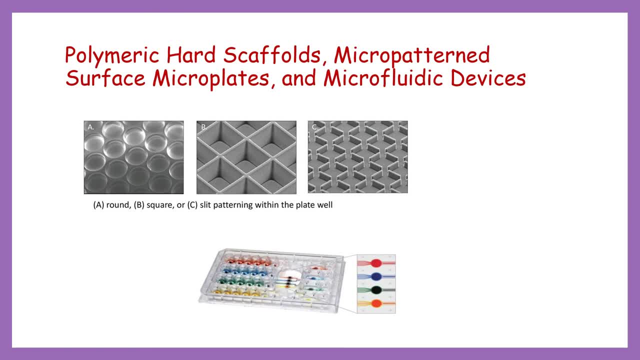 or orthogonally layered polymers are physical supports that can be an inert matrix or engineered tissue on which cells can attach, migrate or fill scaffold compartments to form 3D cultures carrying a geometric configuration. On the other hand, macro-fluidic devices are designed for cell cultures under perfusion. 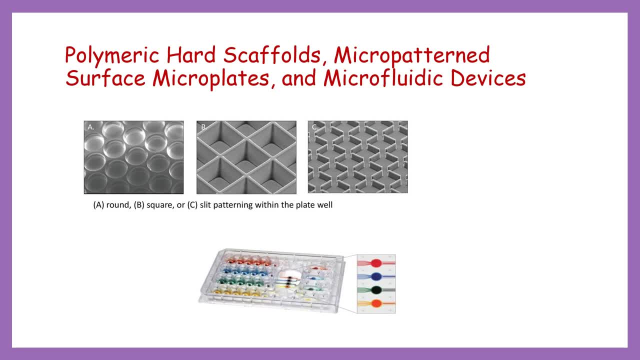 and allow for steady supply of oxygen and nutrients, while at the same time removing waste. Macro-fluidic devices can be built to mimic shear forces found in vivo in cells that are exposed to blood flow, like endothelial cells. A barrier between compartments can be physically incorporated into the device, or it can be. 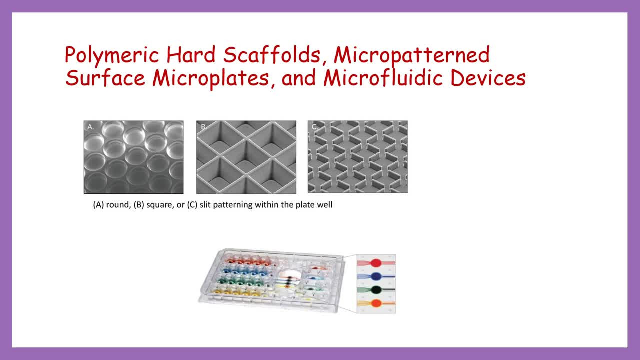 a non-physical barrier, such as a supporting matrix. mimicking ECM Macro-engineering of macro-fluidic devices also allows for the development of organ-on-a-chip platforms with 3D tissue models have been described for a variety of organs, including 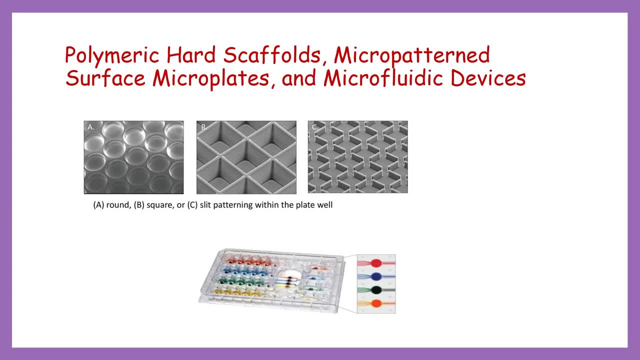 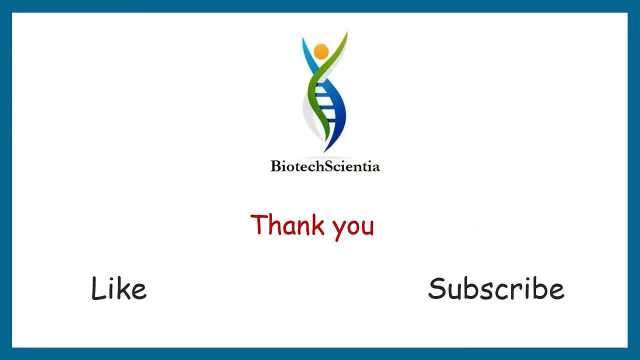 skin, muscle, liver and neural tissues, bridging in vitro cell culture and in vivo animal models. The technologies organ-on-a-chip are poised to provide advanced tools for drug development and high-throughput screening in the future.